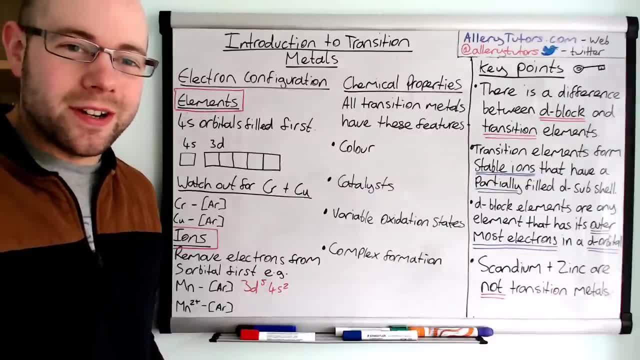 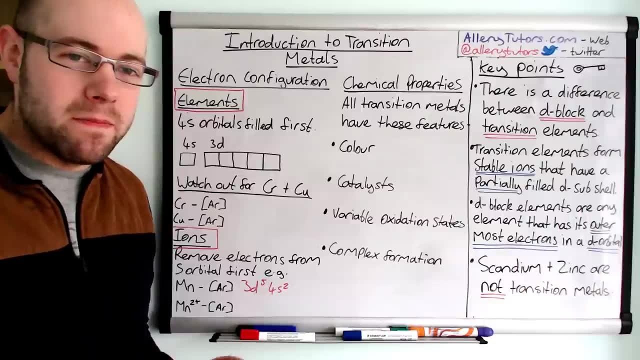 Hi there, my name is Chris Harris and I'm from AllergyTutorscom, and in this video, we're going to be looking at an introduction to transition metals. Now, transition metals are the group of elements that are in the middle of the periodic table. 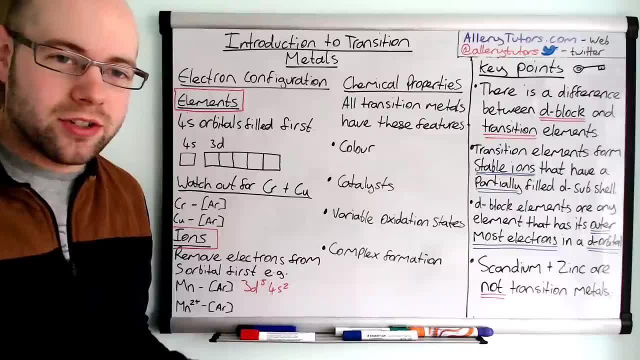 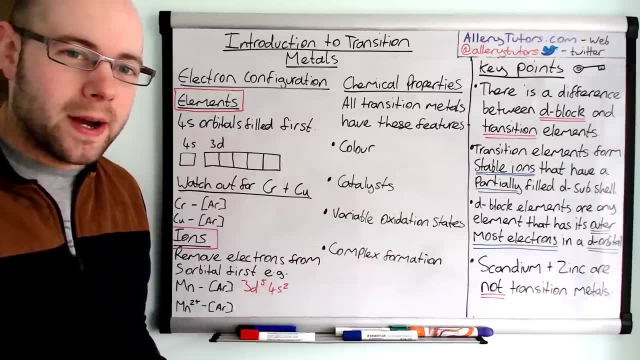 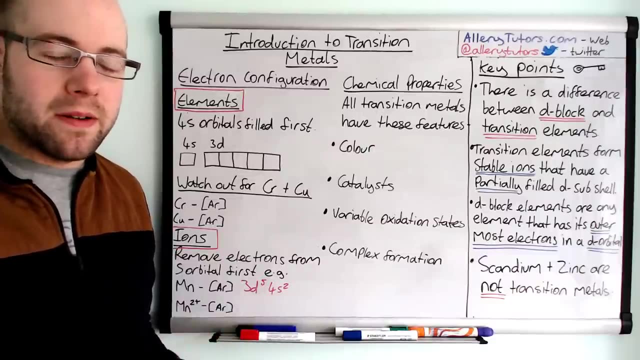 They are, as the name suggests, metals, So they have giant metallic structure, they have high melting points and they can conduct electricity and are good conductors of heat as well. Because of their high melting points as well, some of the metals can be useful for scenarios where you need a large amount of heat. 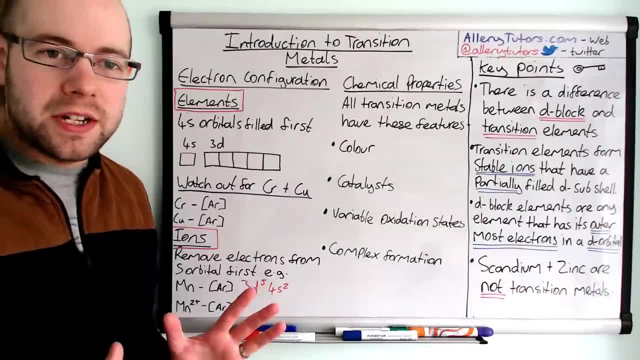 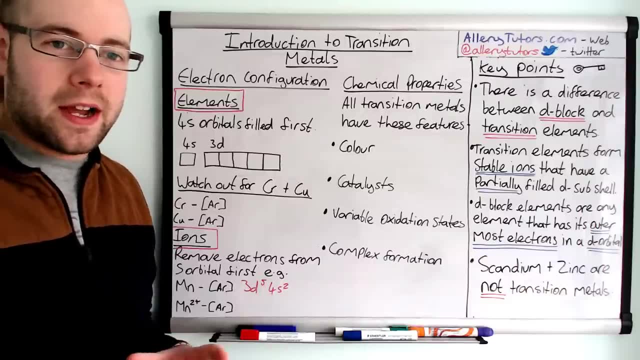 That could be in furnaces and jet engines. You could use titanium, for example, and they also have some strength as well. So, for example, you can use iron to make steel and that can be used to make frameworks for buildings and houses. 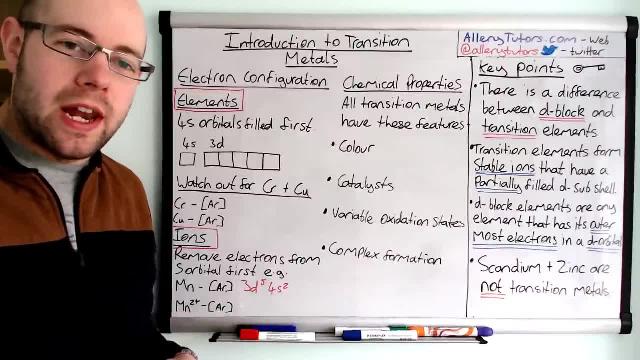 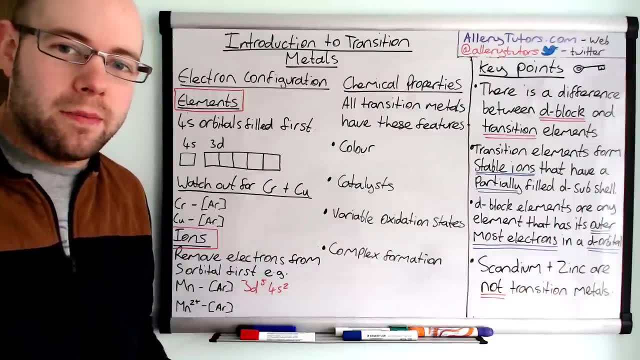 So they're really, really useful. We're also going to look at electron configuration of the elements and the ions that they form. We're going to look at their chemical properties and we're also going to look at some definitions of a transition metal and a d-block element. 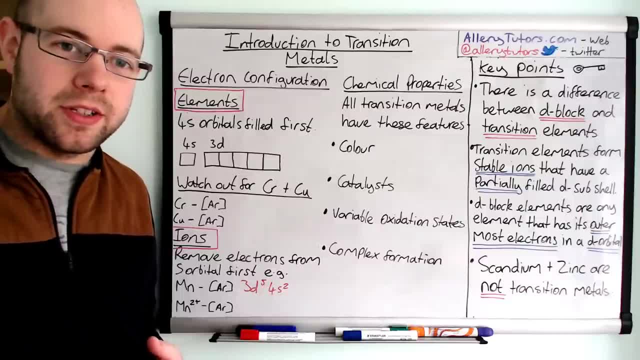 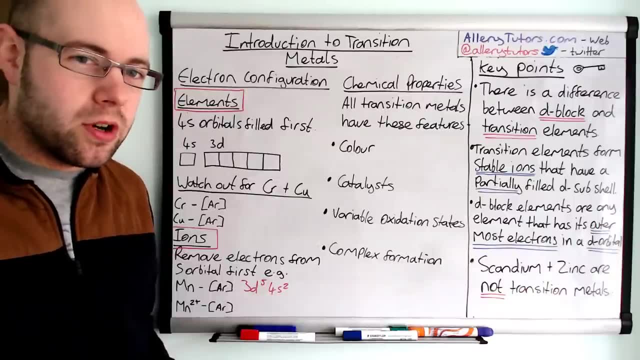 Because it is important that we need to know the difference between them, And that's where I'm going to start. So over on the right hand side, there we can see we've got the difference between a d-block element and a transition element. You've got to know the difference between these two. 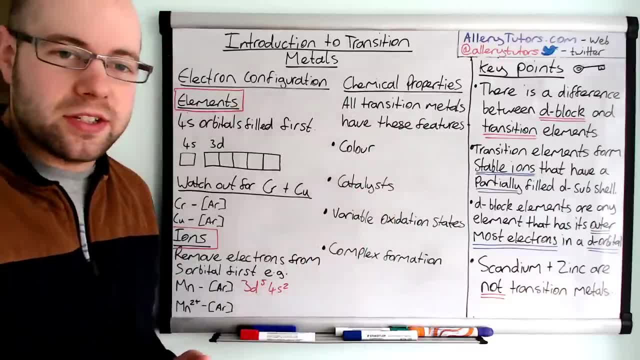 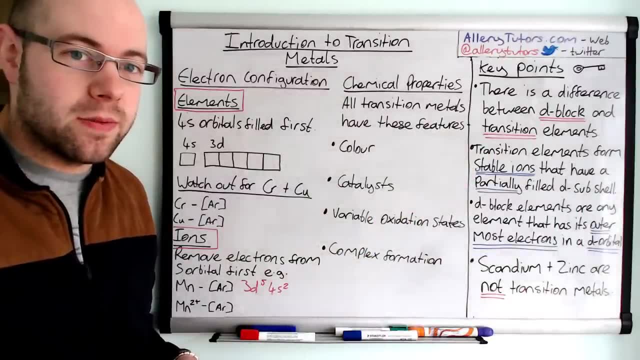 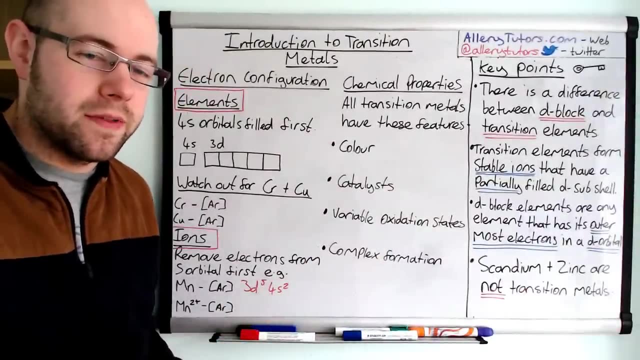 Essentially, a transition element is defined as something that will in a stable ion that forms a stable ion That will have a partially filled d-sub-shell, And that's really important and the ion bit is important as well. We're not talking about the elemental version of the transition metal that has a partially filled d-sub-shell. 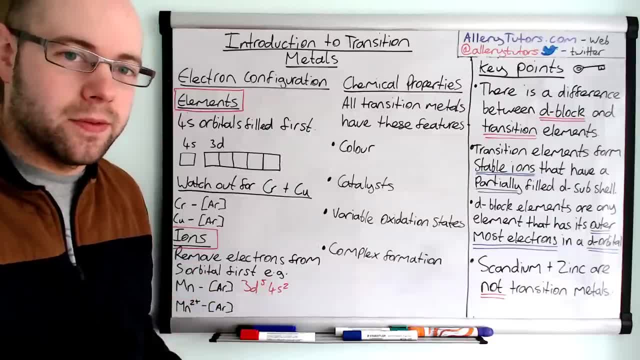 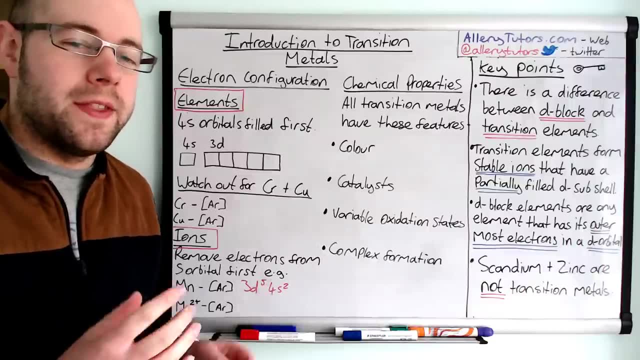 It's the ion, a stable ion, that that transition metal can form. And if that stable ion has a partially filled d-sub-shell, then it will be classed as a transition metal, And this is different to what we call a d-block element. 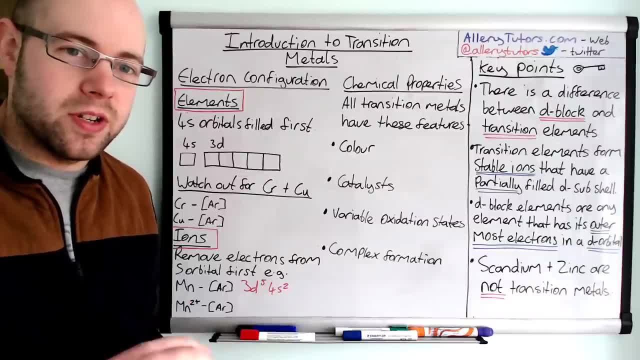 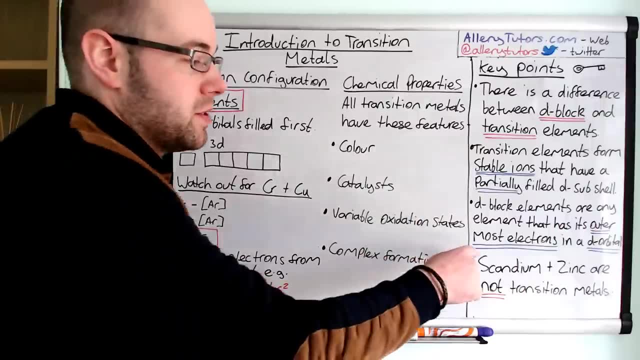 Where this is any element that would have its outermost electrons, In other words the hat At its highest energy level, that occupy d-block or occupy d-orbital, And so we can come up with these two different types of elements. So we have scandium and zinc. 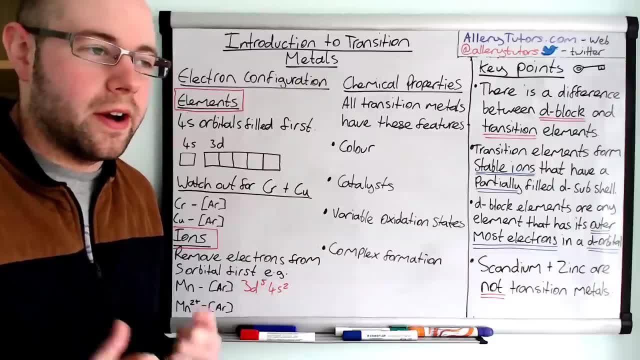 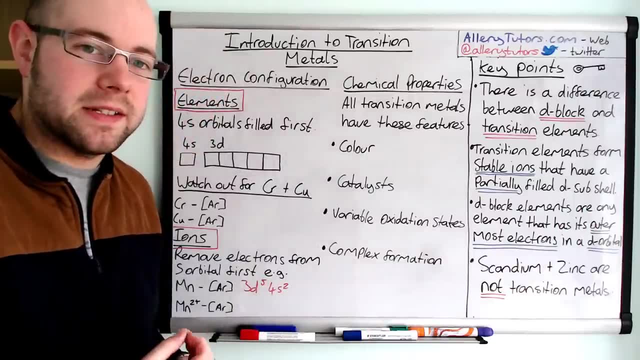 And scandium and zinc are classed as not transition metals. They are either side of the top row of the transition metal block. And scandium, for example, its stable ion is SC3+. Now if we take three electrons away from a scandium atom, 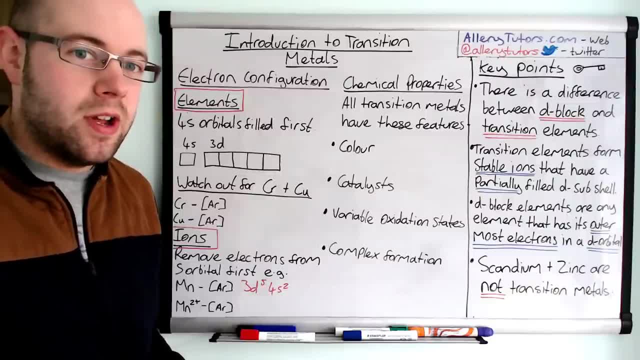 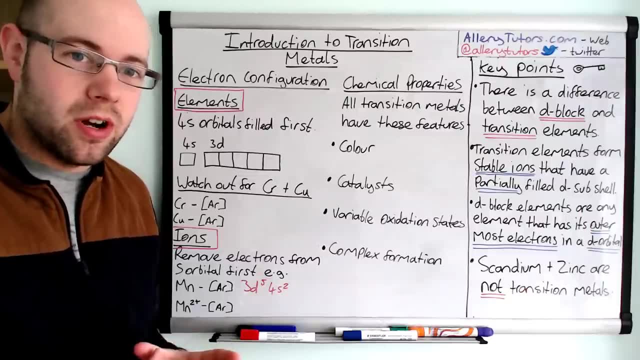 we're left with an ion that has an electron configuration With no electrons in the d-orbital. So because that is not partially filled, we say that scandium is not a transition element, And that's really important that you've got to know the difference between the two. 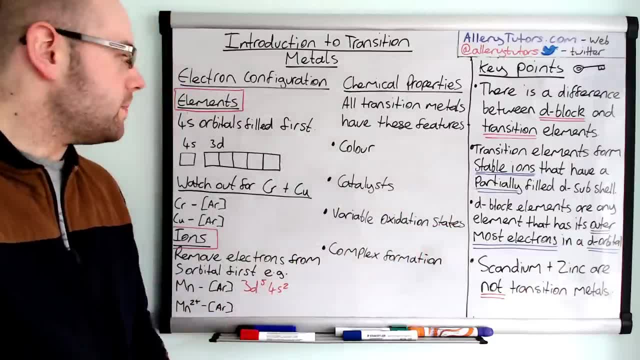 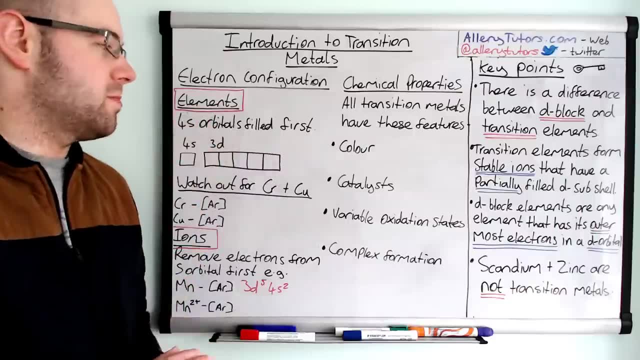 As it's quite a common question for them to ask in the exam. Okay, if we come on to electron configurations Now, electron configurations of elemental transition metals. They always have electrons in the 4s orbital And some of them are filled. 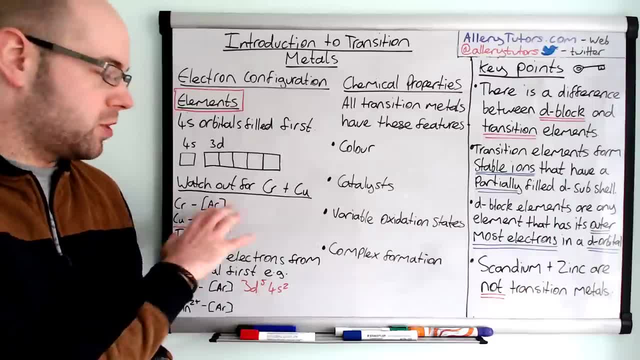 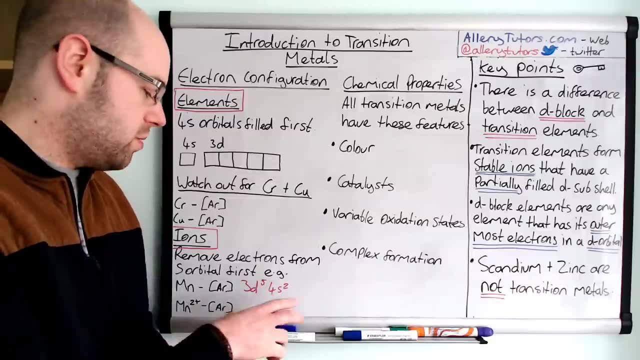 So they have two electrons in there, And some of them are not, which we'll come on to in a minute as well. There is some exceptions, But I'm just going to go through and show you how we can fill these up And show you what the electron configuration is as well. 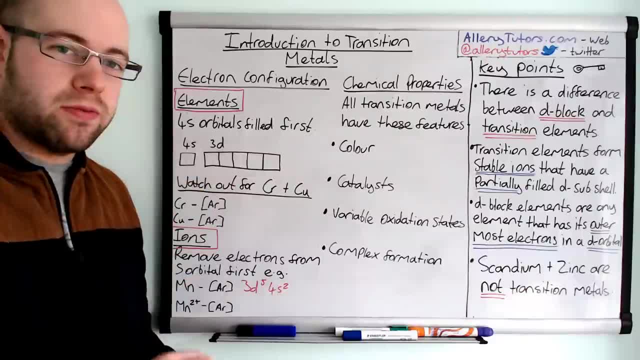 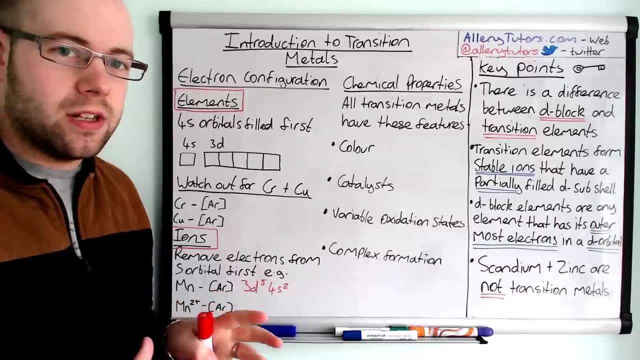 Now these things. I've drawn the 4s and 3d in the same row, So there's no energy difference here. But the 4s and 3d orbitals are actually really close together in terms of energy, And that's why we've got the word transition there as well. 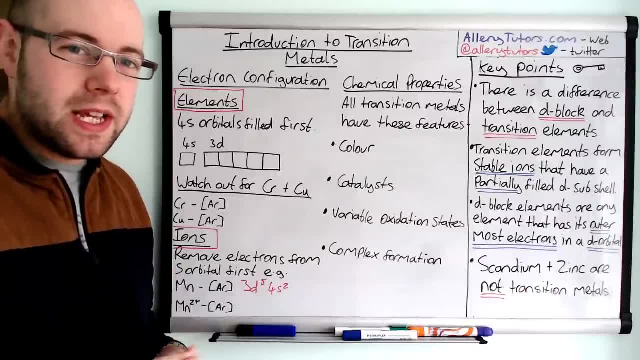 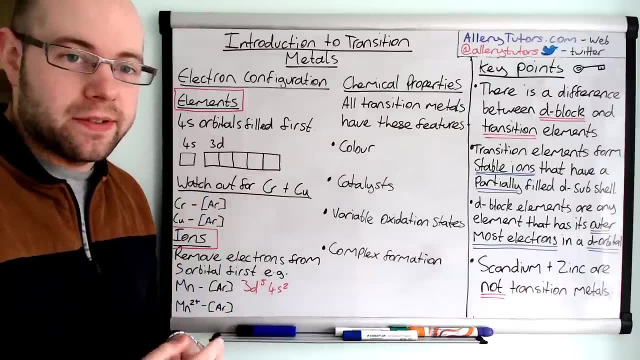 Because the electrons can move Relatively easily between the 4s and the 3d orbitals, And these orbitals can change in terms of energy, Energy levels as well. So we're going to start with the first element in the transition. 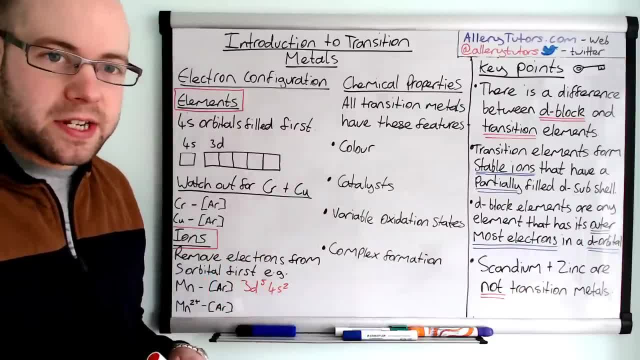 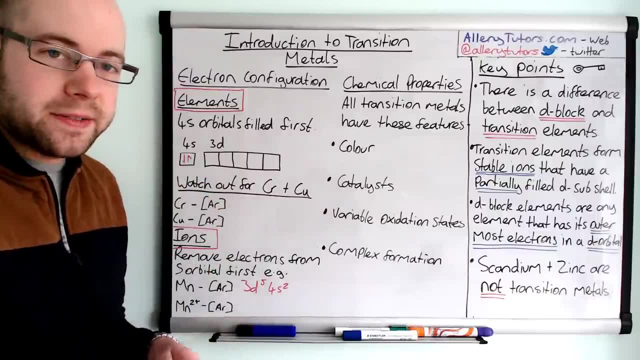 Well, in the d block, should I say, Which is scandium? Now, scandium has two electrons in the 4s orbital, So I'll draw them there, And it also has one electron in the 3d orbital. Remember, we're talking about elements here. 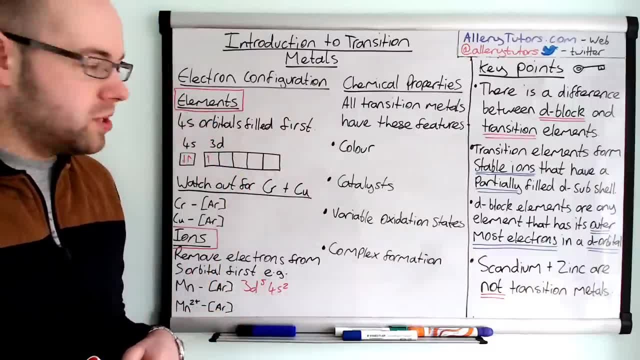 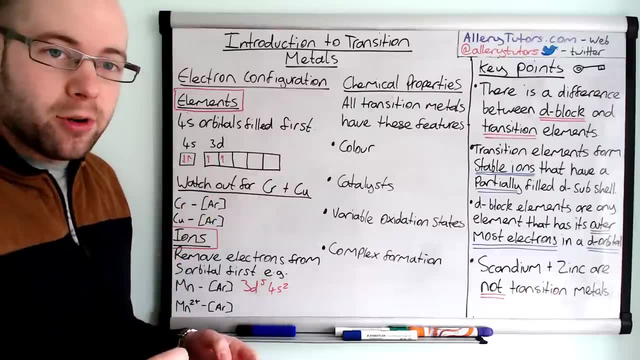 So we're not talking about the ionic version. If we go next along to titanium, Titanium would have one electron in the next orbital. Remember, we can't put the electron in the same orbital because of electron repulsion, So they sit in a separate orbital. 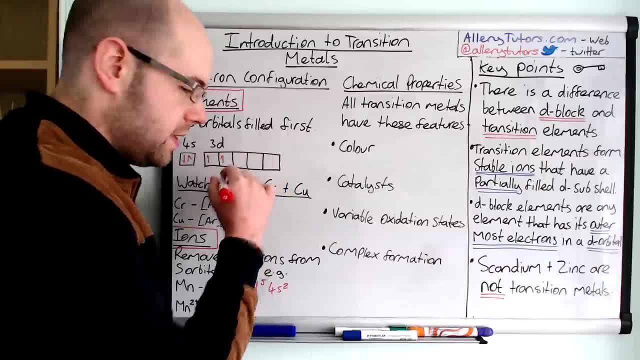 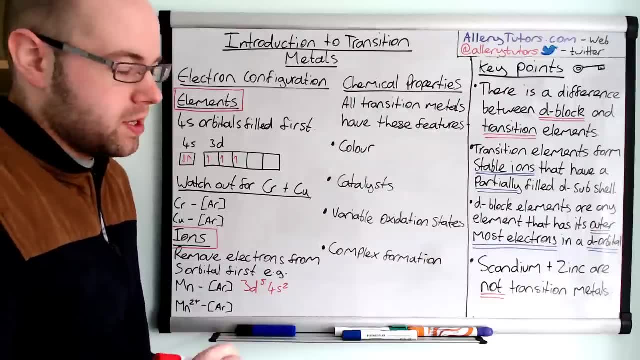 If we come on to the next one, which is titanium- Sorry, vanadium. So vanadium has got three electrons in there. And then if we come to chromium- Now this is where it gets a little bit different. You can see, here with chromium we've got four electrons here. 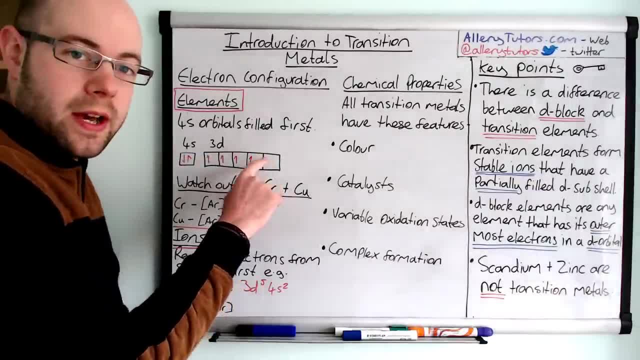 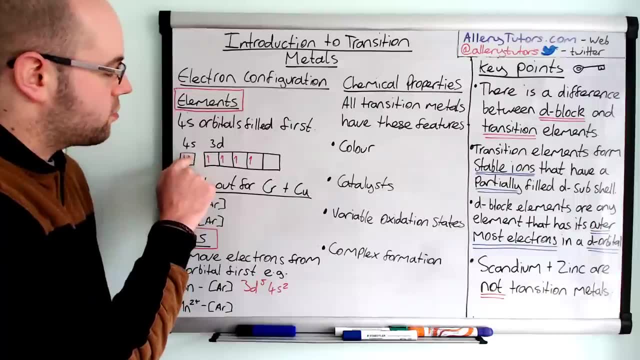 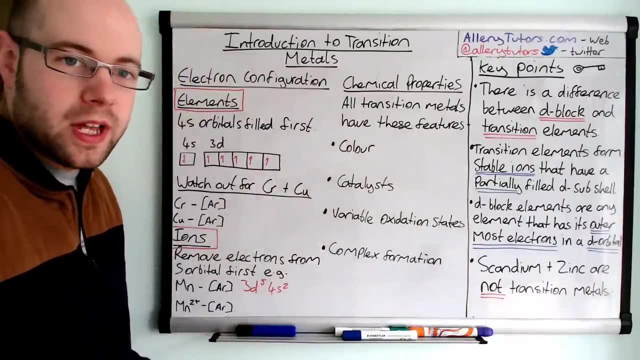 However, what happens is to get half filled. d subshell is actually quite stable And what chromium does, or the electron configuration of chromium, Is this electron in the 4s orbital can actually occupy this spare orbital in the d subshell. So what we have effectively for chromium: 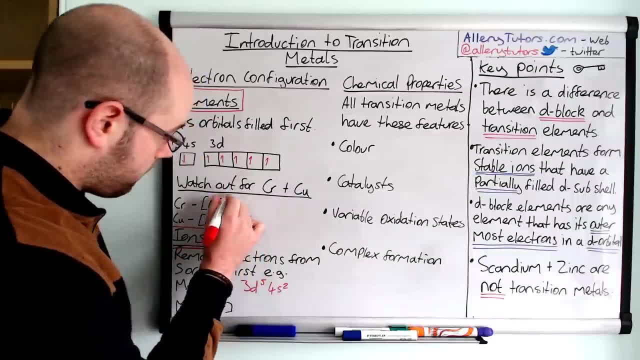 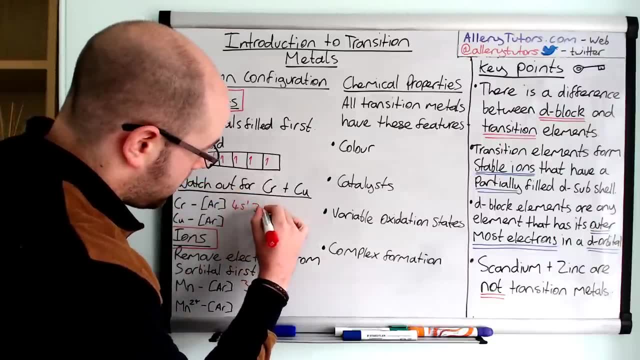 And you've got to be really careful, for this Is actually: we have the configuration for argon, which is here, And we have 4s1. Which we'll put there, And we have 3d5. And it's important to know that. 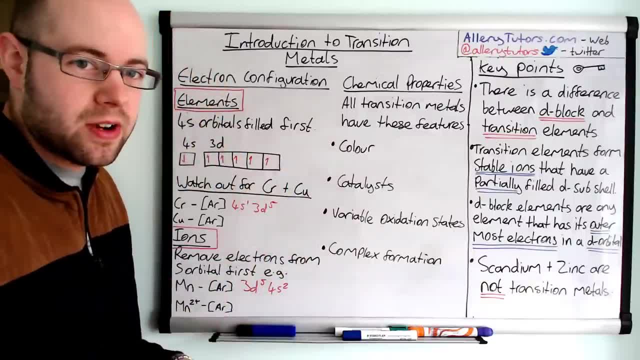 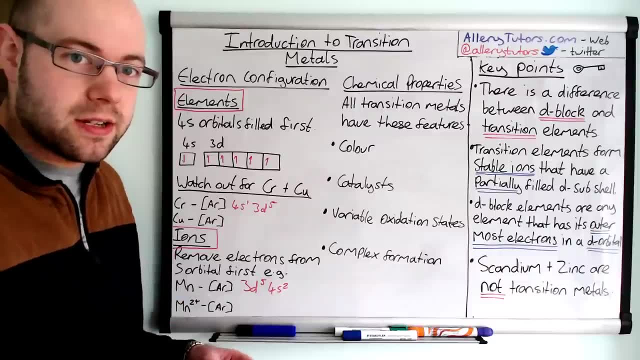 That chromium is one of these ones, a little bit strange, A little bit different, And the reason why it does this is because this Configuration, having a half filled 3d subshell, is a lot more stable than not having that. Okay, If we go to the next element, which is manganese, 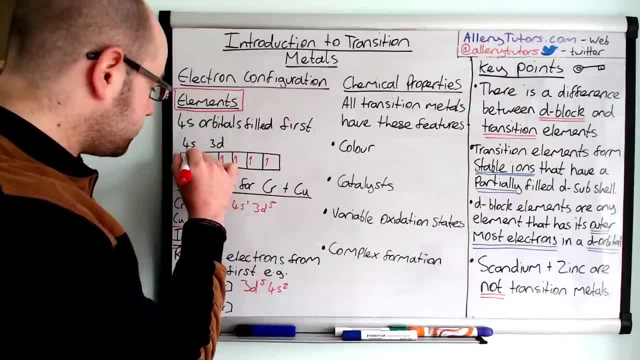 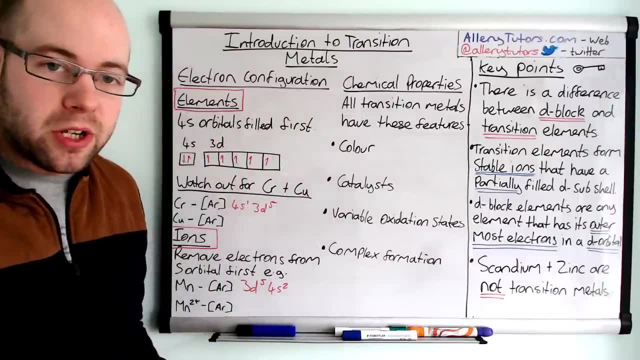 Now, manganese will fill up this electron here first. So remember s1.. So remember s orbitals will fill up first. So manganese has that configuration. The next one along is iron, And iron would then start and fill up the d, The d electron. 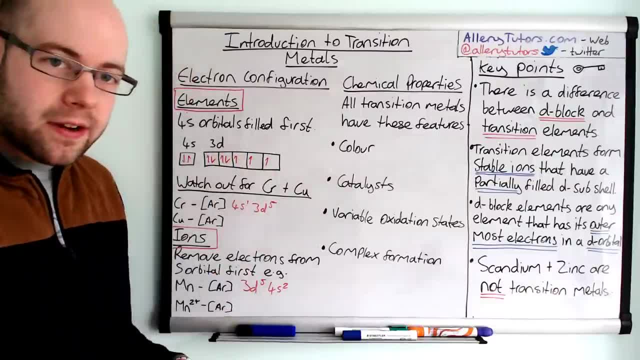 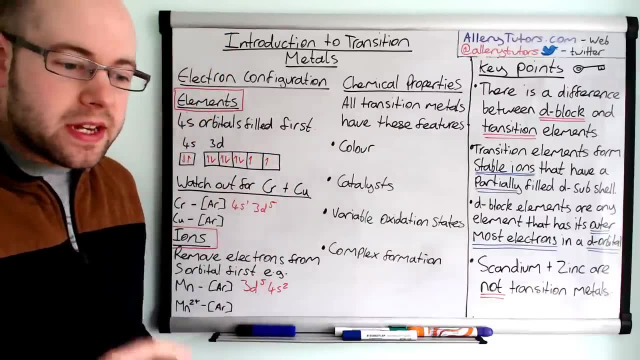 The next one after that is cobalt, And again, cobalt would have that configuration. The next one along is nickel. Nickel will have this configuration here, And the next one along would be copper. Now, copper does a very similar thing to what chromium did. 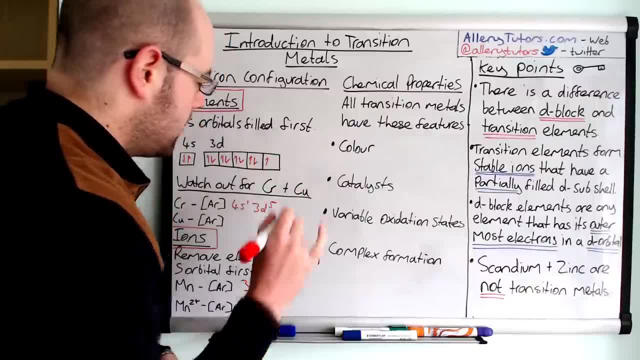 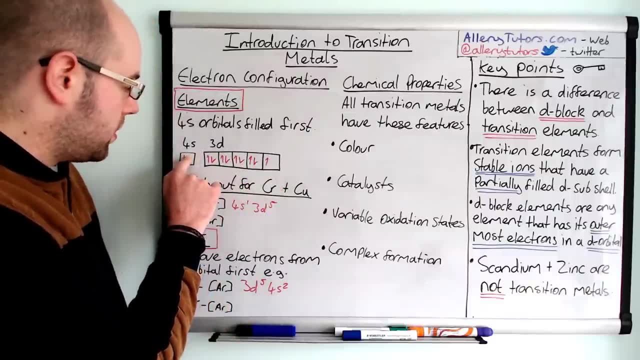 It's one of these bizarre ones, So we'll add the extra electron for copper there. But again, to form a full d subshell is more stable than leaving it like this. So the electron from the 4s orbital here will then move into this orbital. 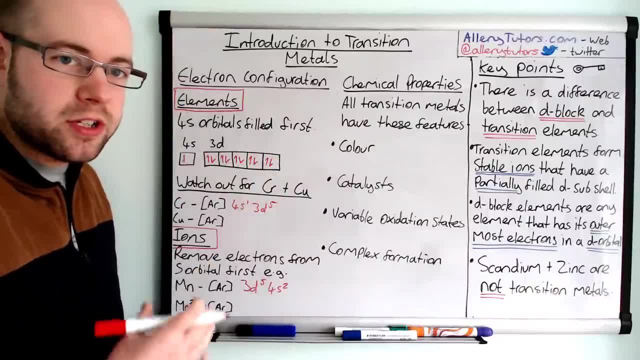 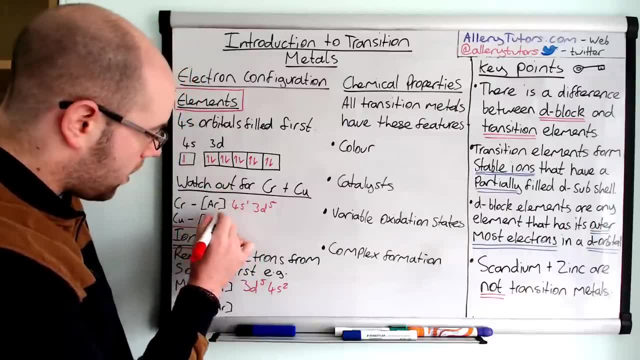 And now we have a full 3d subshell which is more stable than the configuration that we had before. So for copper, the configuration is the configuration for argon, And it will be 4s1.. And then 3d10.. 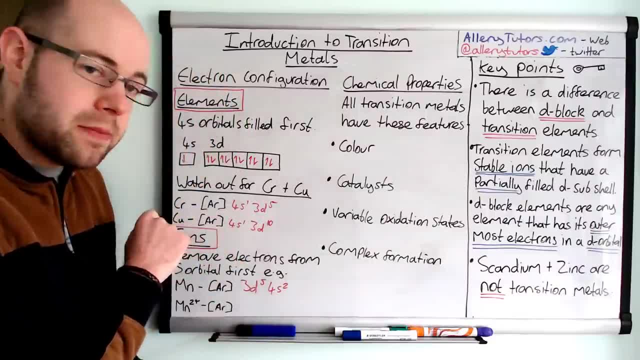 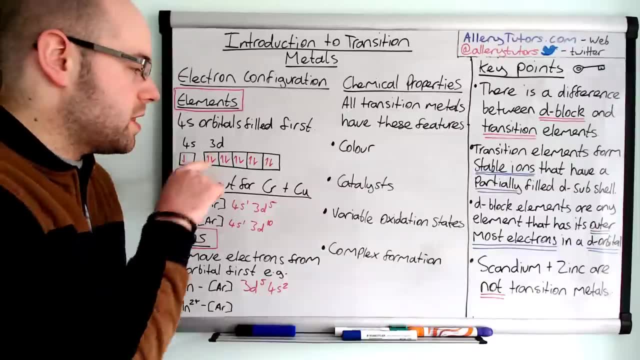 So you can see that we have a 4s1.. And these are the only two elements in the transition metal block in that first row that actually have one electron in the s orbital when they're an element. And if we come onto the last one, 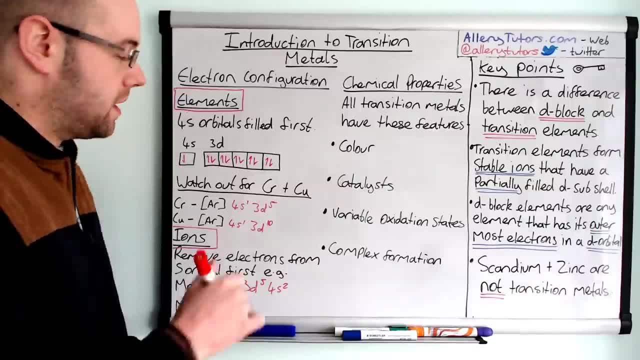 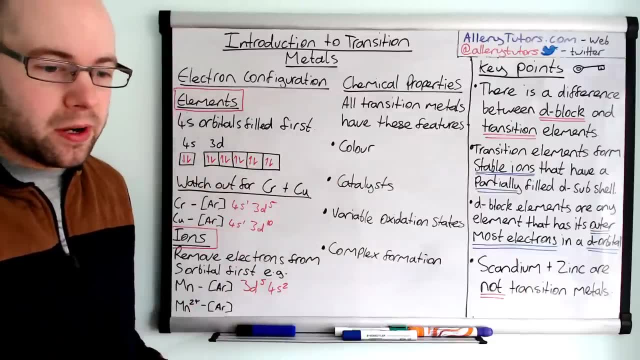 The last one, there was zinc. That's the last element after copper. Obviously, the electron for zinc will go into that s orbital and then it's full, And after this we then go into the p block, which would be gallium, which would be next after that. 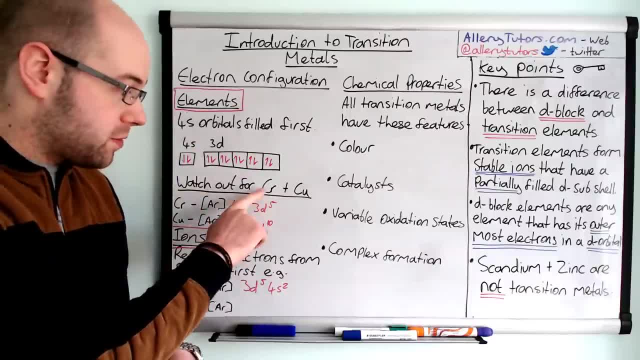 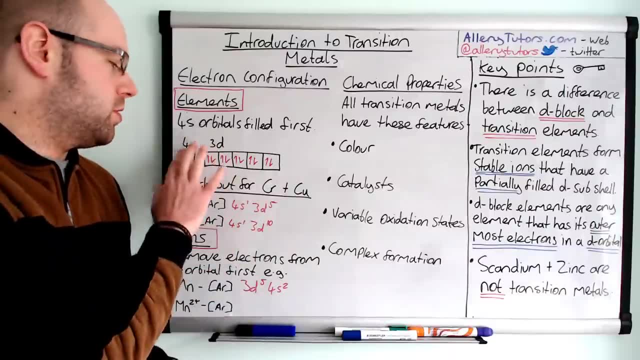 So that's effectively how we fill them out. But you do have to watch out for that. You do have to watch out for chromium and copper, As these do have this different electron configuration to the standard one. All the other elements have two electrons in the 4s orbital. 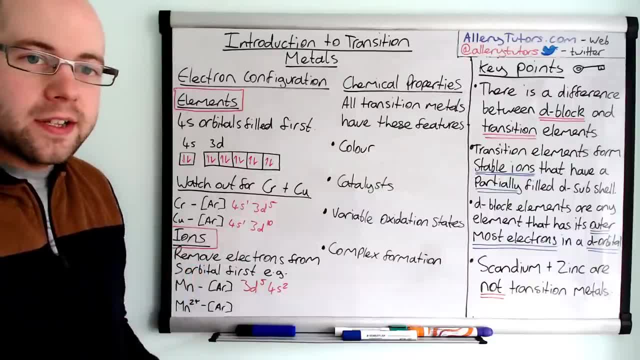 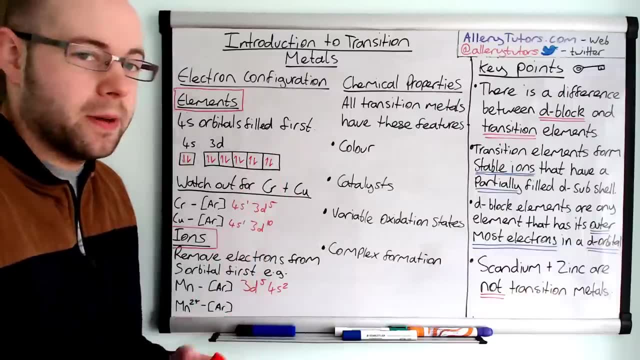 Okay, If we just go into the one down here. These are ions, So it's very common for transition metals to lose electrons as well. It gives them this difference in oxidation state, which we'll come onto in a minute for the properties, But we remove electrons from the s orbital first. 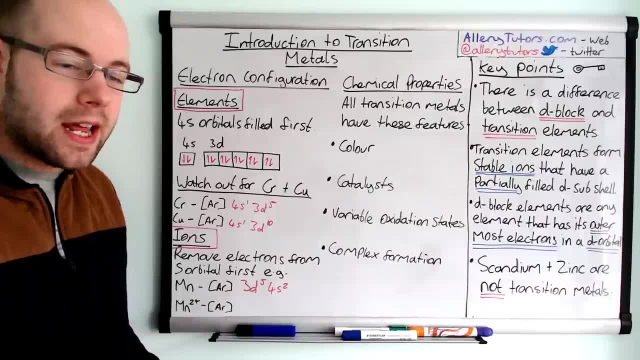 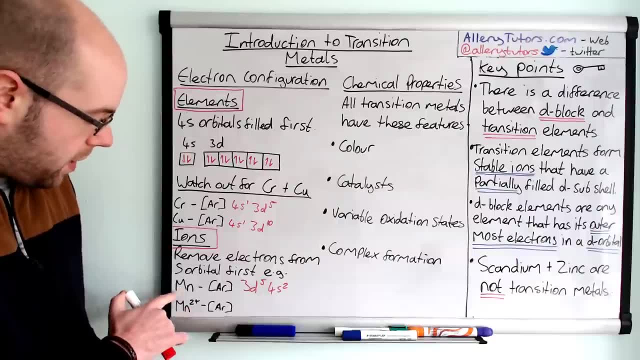 And that's because the s orbital is actually slightly higher, Higher in energy than the d orbital when we're removing electrons. So we remove it from there first because it's easier to remove. So if we look at this, for example, we've got manganese as an element here. 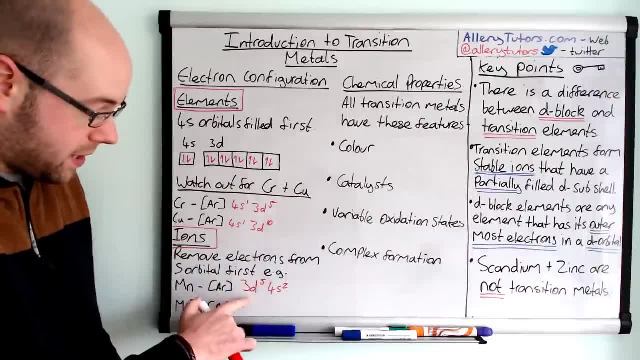 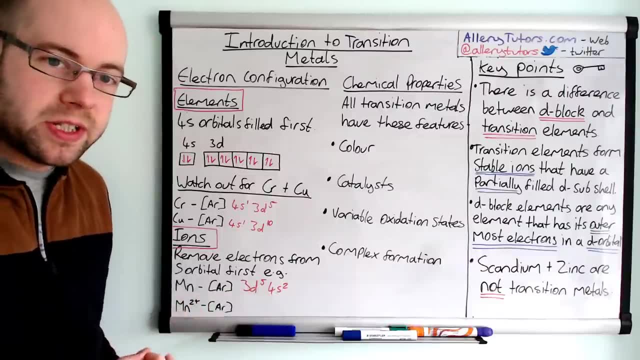 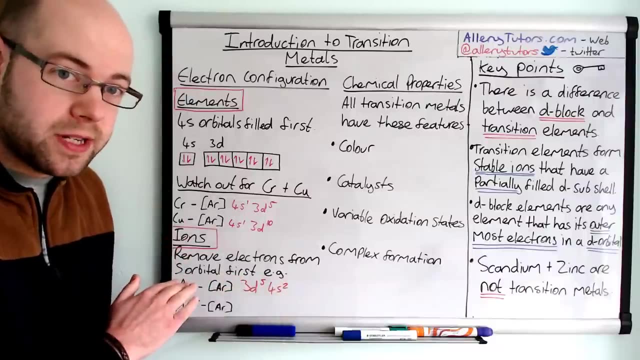 The atomic or the elemental manganese is. 3d is the configuration for argon 3d5, 4s2.. Manganese, though, can come in. one of its stable ions is Mn2+, And we effectively remove the 4s electrons first, before the 3d. 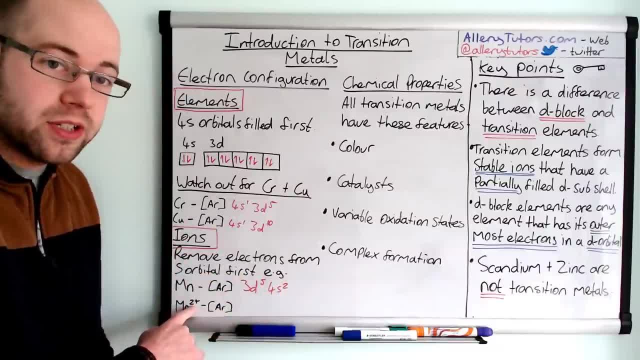 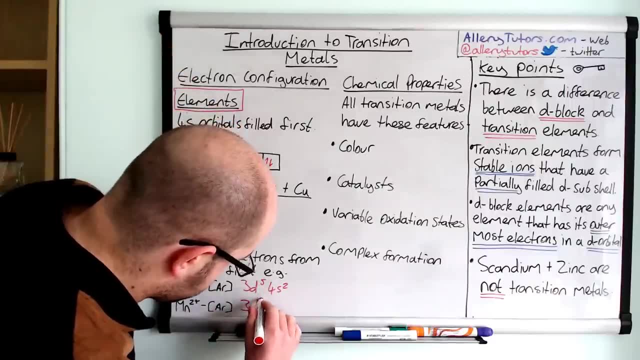 And so effectively we only need to remove two electrons. because it's Mn2+, They get removed from the 4s first And effectively what we're left with is 3d5.. Once you've removed the electrons from the 4s, 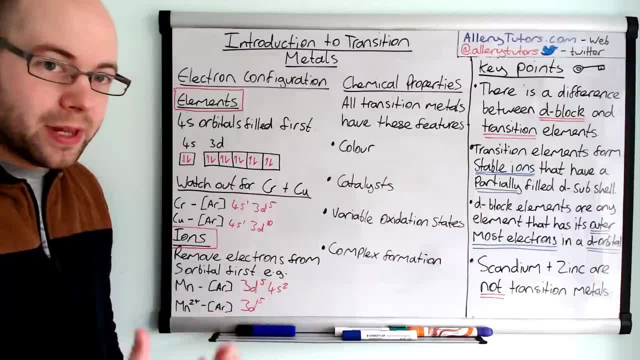 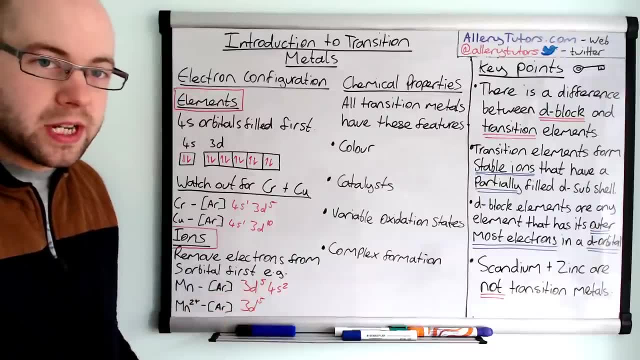 If you have, say, for example, a 3 plus ion, For example iron, So Fe3+, You would remove the electrons from the s orbital first. Then you'd remove an electron from the d orbital. But it is really important you always remove electrons from the s orbital first. 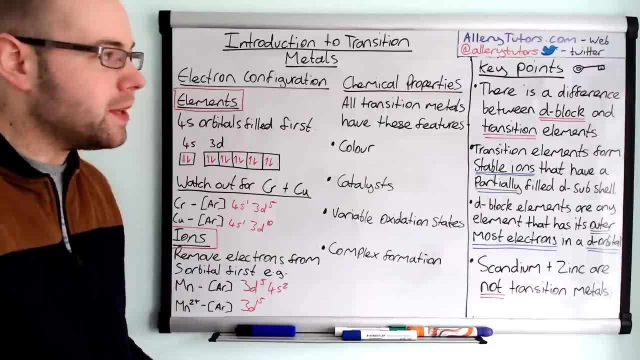 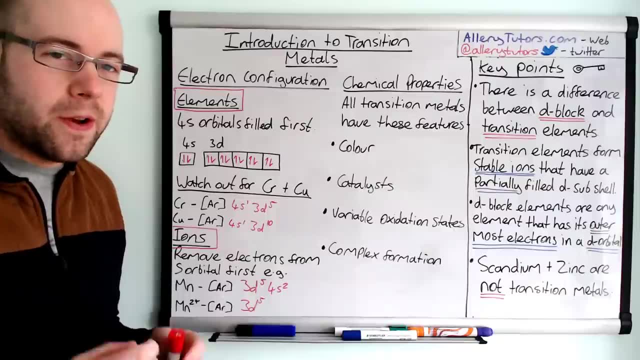 Before the d orbital. That's really crucial. Okay, just coming on to the last bit, Just looking at some chemical properties of transition metals. They all have certain things in common: They're really useful in industry, in particular For things like catalysts and paints, etc. 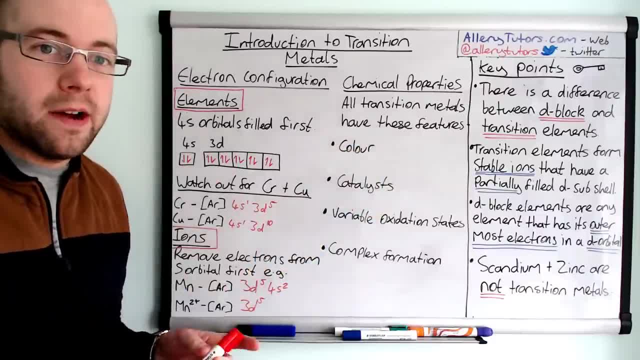 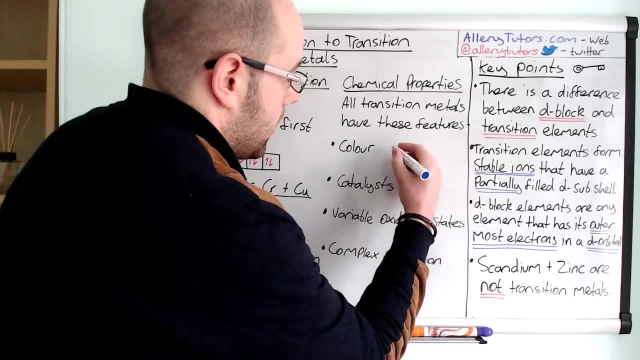 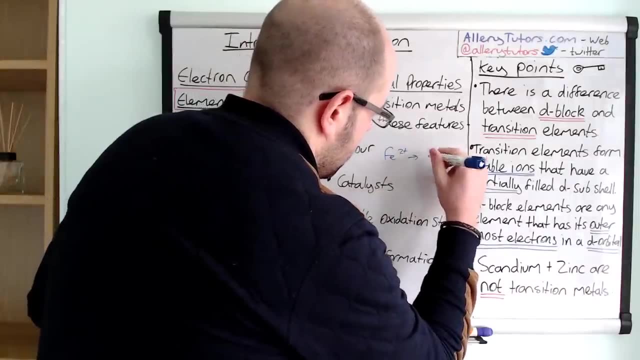 So one of the features of a transition metal is colour. Now, for example, we can give an example for colour, And we'll do this one in blue. For example, you might have iron, So we'll put that Fe2+, For example. we'd have a green colour. 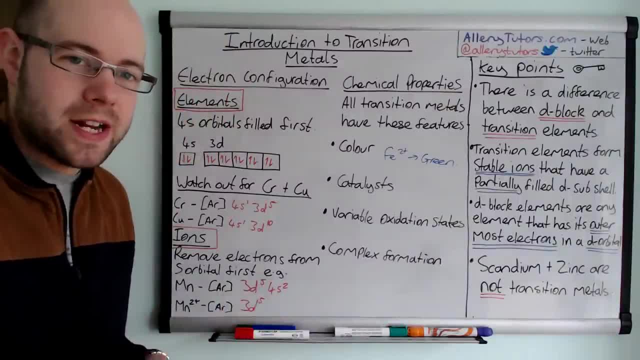 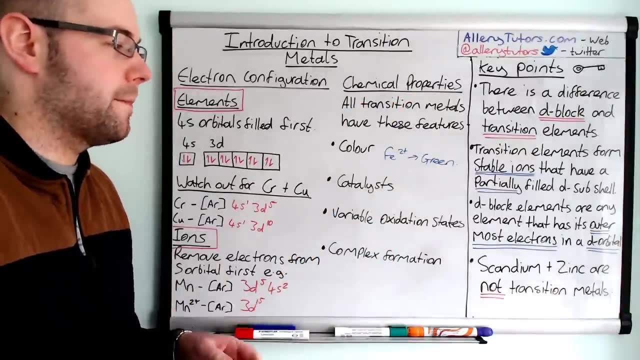 Fe3 plus might be a red, Like a reddish orange colour, etc. So a lot of these transition metals are colourful metals. So it's really nice to look at Catalysts. They're really good catalysts. For example, we can use iron as a catalyst in the Haber process. 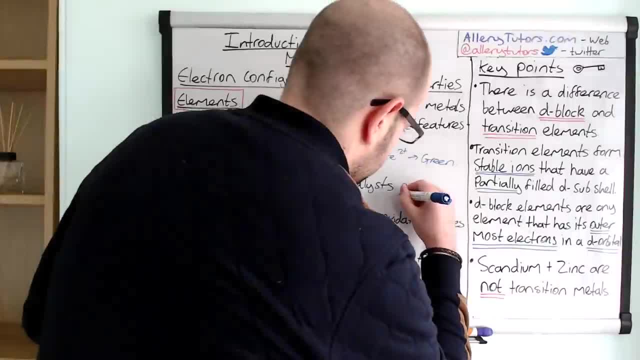 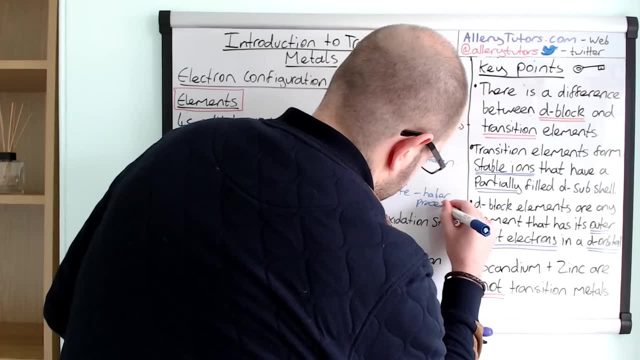 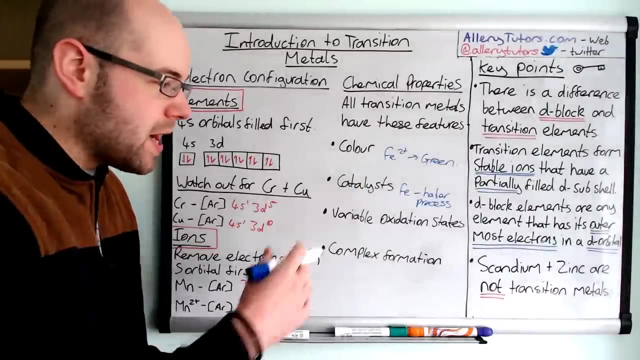 In the manufacture of ammonia. So we'll put that in there. Put Haber process, There we go. And there are loads of other catalysts as well, But that's just one example. Variable oxidation states: Again, the word transition means they can vary the oxidation states. 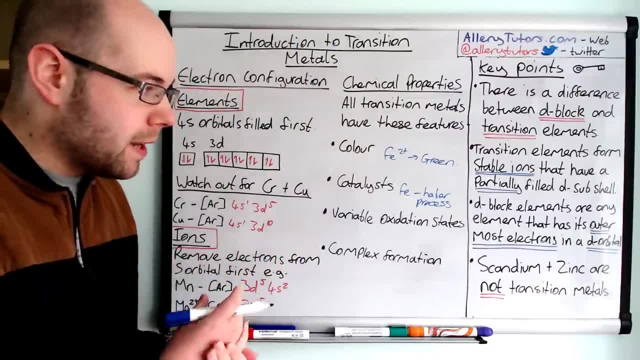 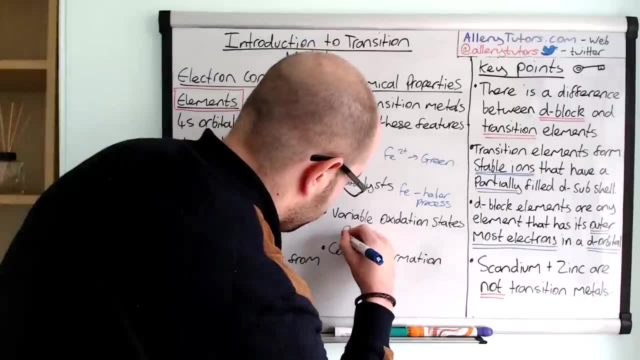 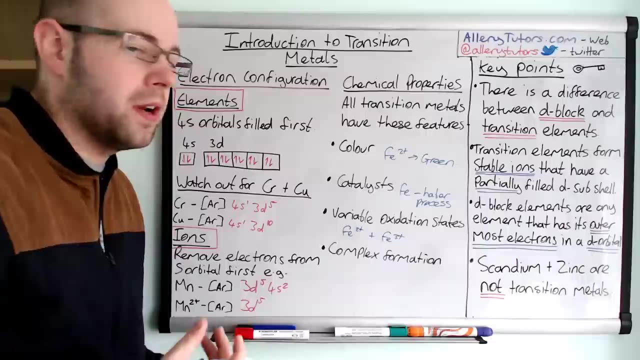 And that makes them useful for potential reducing and oxidising agents as well. So, for example, you could have Fe2+ And you can have Fe3+. So there's just one example of a transition metal that has a different, same element. So same number of protons. 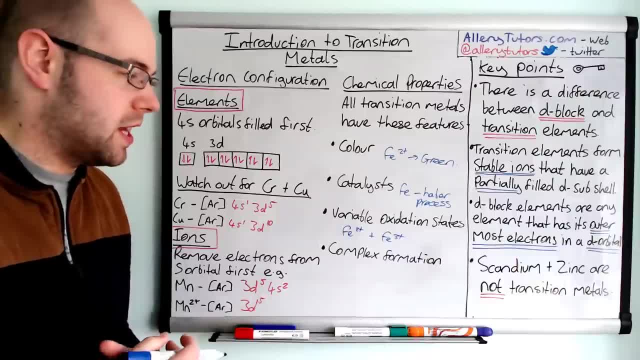 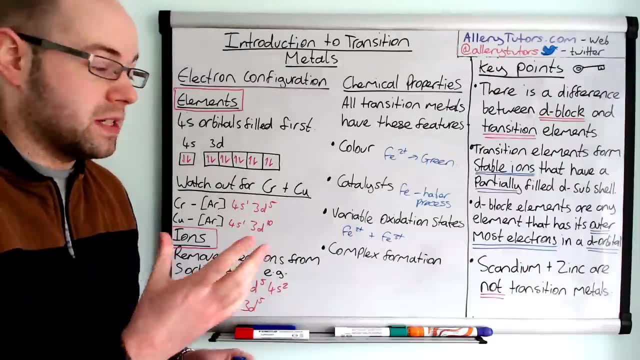 But it's got a different oxidation state. It's got a different number of electrons in that outer shell And the last one is complex formation. Now, complexes are a transition metal. Basically it's a large molecule with a transition metal in the middle. 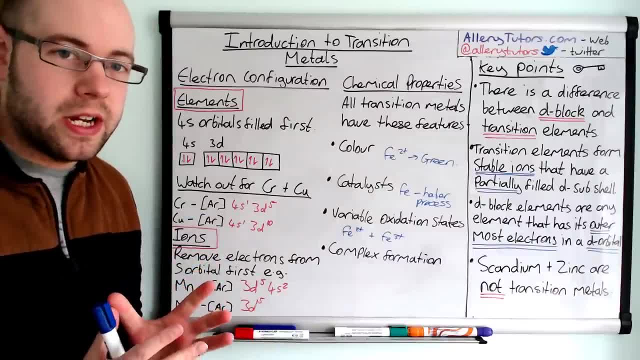 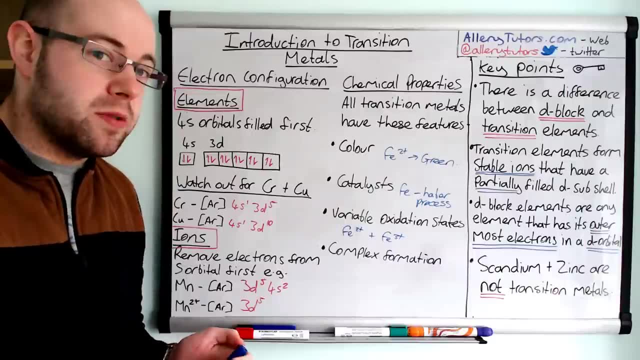 And we have ligands that surround it And they're datively covalently bonded, Or co-ordinately bonded, To the metal ion in the middle, And transition metals have this very unique ability to form large complexes. So, for example, you might take